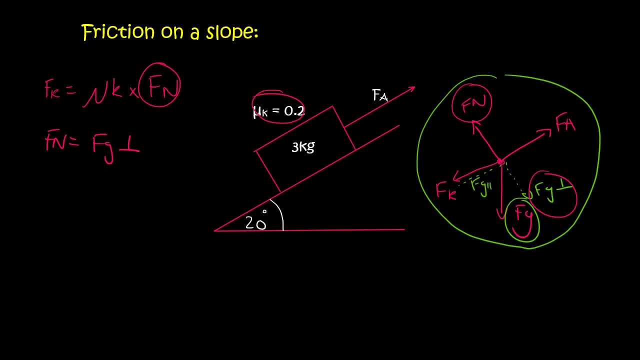 perpendicular. Now in the previous question I showed you that FG perpendicular is equal to MG cos theta. So can you see how this works? Friction is equal to this- funny symbol- times by normal force. But then normal force is equal to that and that is equal to this. So if we just substitute- 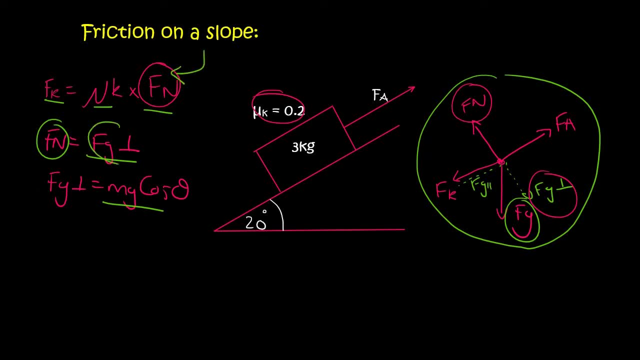 the normal force, we get this. So if we know that this normal force is equal to FG perpendicular, but we also know that FG perpendicular is equal to this, then we can take this part and just put it over there. And so friction kinetic is going to be equal to the funny symbol multiplied by MG cos. 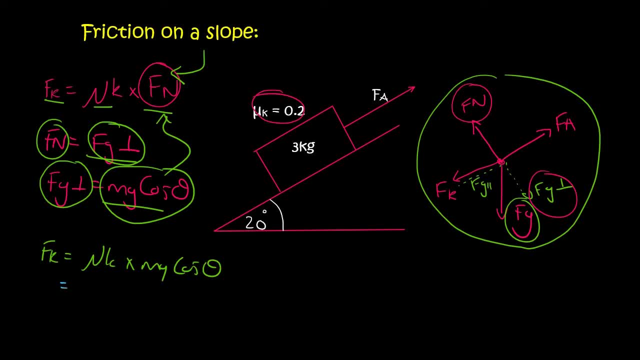 theta in a situation like this. And so now we can fill in the symbol as 0.2.. Your mass is 3 and your gravity is 9.8.. And then it's cos of 20. And then we can just type all of that in on the calculator and you end up with 5.53 newtons. That 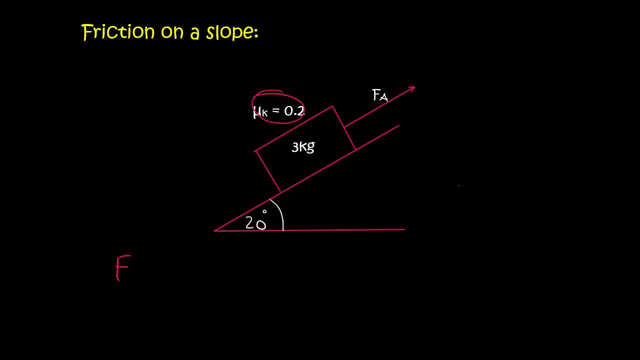 is your friction. So let's do that a little bit faster. So we know that friction kinetic is equal to the coefficient multiplied by normal force. Now normal force is equal to. it's the same as your perpendicular, and your perpendicular is MG cos theta. So we can take this and put it in the 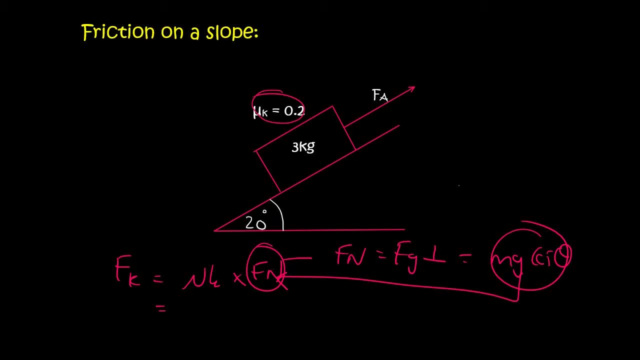 place of normal force. And so your kinetic friction is just going to be equal to 0.5.. So that's 3 multiplied by 9.8 times by the cos of 20.. And so, guys, I've changed the values for this. 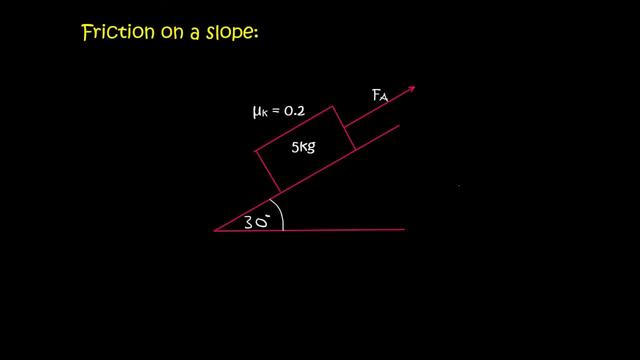 question. Now I've updated everything. Have a go and see how quickly you can work out friction and then play the video again and see if you got it correct. So we know that friction kinetic is equal to the coefficient multiplied by the normal force. Now we can go do a free body diagram. 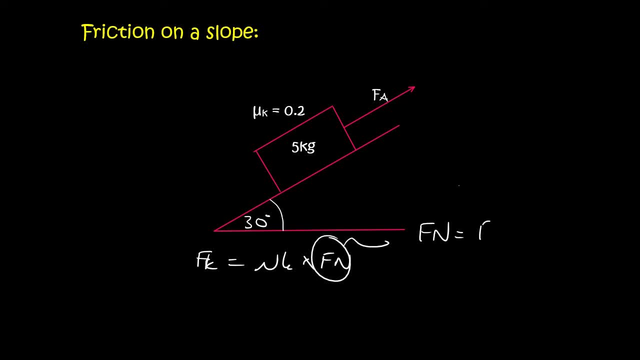 but we know that normal force on a slope is equal to FG perpendicular. Now we know that FG perpendicular is equal to MG cos theta, So we can replace this normal force with MG cos theta, And so that's going to be equal to 0.2 multiplied by the mass, which is 5. 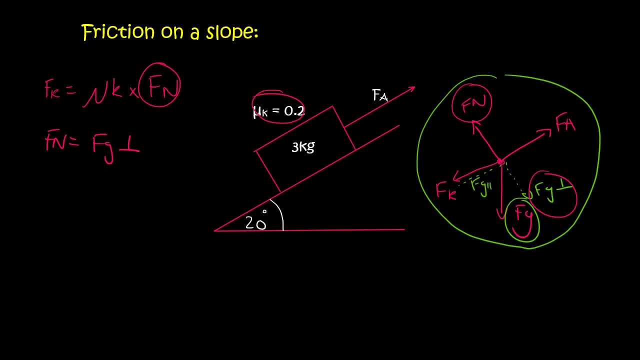 perpendicular. Now in the previous question I showed you that FG perpendicular is equal to MG cos theta. So can you see how this works? Friction is equal to this- funny symbol- times by normal force. But then normal force is equal to that and that is equal to this. So if we just substitute- 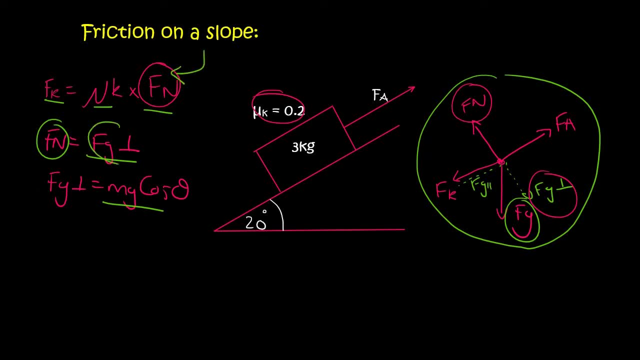 the normal force, we get this. So if we know that this normal force is equal to FG perpendicular, but we also know that FG perpendicular is equal to this, then we can take this part and just put it over there. And so friction kinetic is going to be equal to the funny symbol multiplied by MG cos. 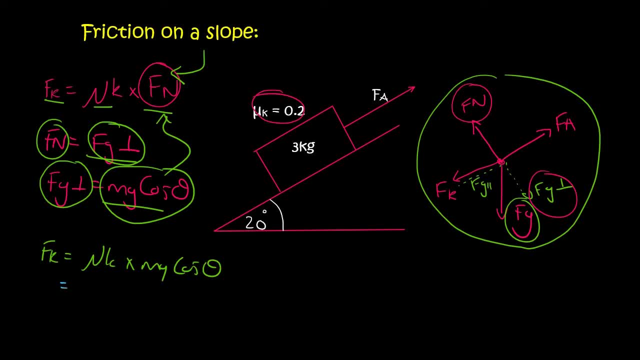 theta in a situation like this. And so now we can fill in the symbol as 0.2.. Your mass is 3 and your gravity is 9.8.. And then it's cos of 20. And then we can just type all of that in on the calculator and you end up with 5.53 newtons. That 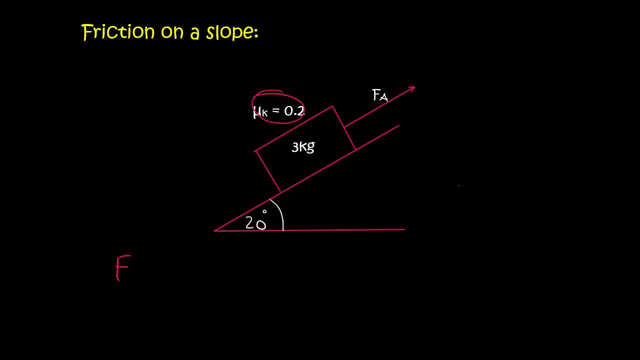 is your friction. So let's do that a little bit faster. So we know that friction kinetic is equal to the coefficient multiplied by normal force. Now normal force is equal to. it's the same as your perpendicular, and your perpendicular is MG cos theta. So we can take this and put it in the 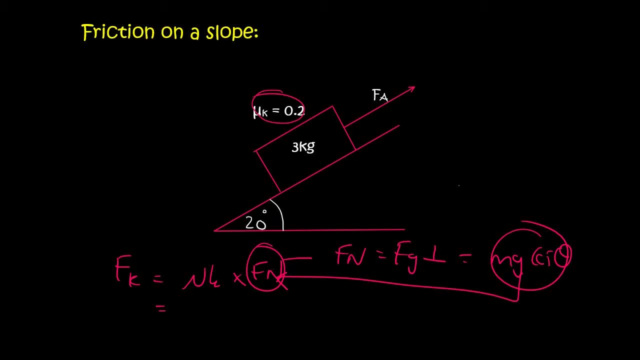 place of normal force. And so your kinetic friction is just going to be equal to 0.5.. So that's 3 multiplied by 9.8 times by the cos of 20.. And so, guys, I've changed the values for this. 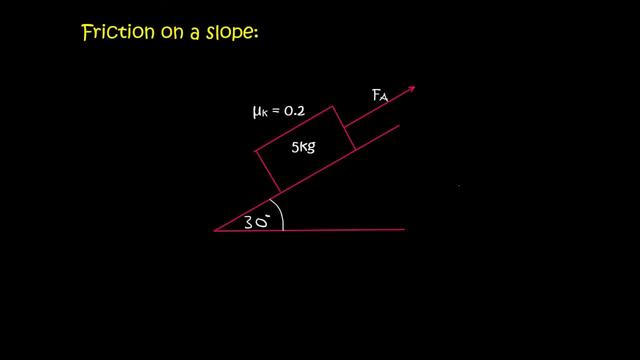 question. Now I've updated everything. Have a go and see how quickly you can work out friction and then play the video again and see if you got it correct. So we know that friction kinetic is equal to the coefficient multiplied by the normal force. Now we can go do a free body diagram. 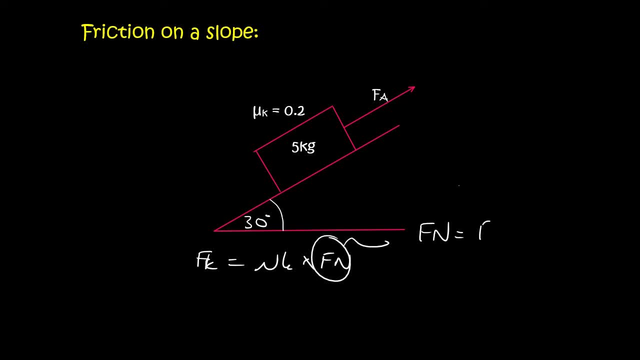 but we know that normal force on a slope is equal to FG perpendicular. Now we know that FG perpendicular is equal to MG cos theta, So we can replace this normal force with MG cos theta, And so that's going to be equal to 0.2 multiplied by the mass, which is 5.